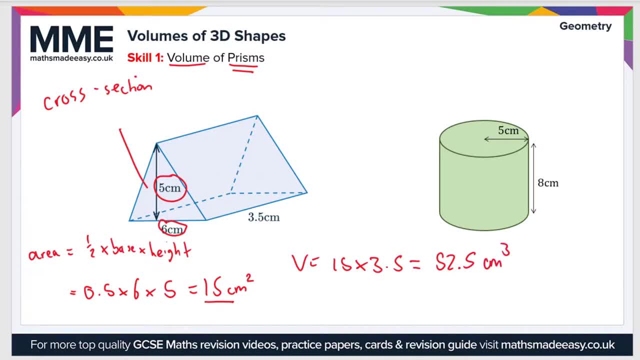 in centimetres cubed in this case, because the values in the question are given in centimetres. So let's have a look now at this cylinder here. So a cylinder is essentially just a circular prism. So in order to calculate the area of the cross section, we'll use the area of a circle, which 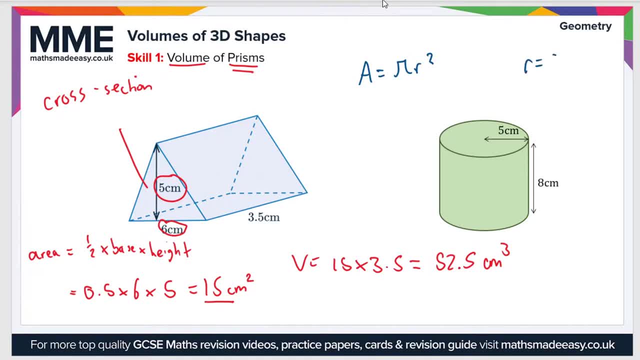 is pi. r squared Now, r equals 5, that's this radius here which is 5, so if we put that into the formula, then that gives us 5 squared, 5 squared times pi. so the area is 25pi. 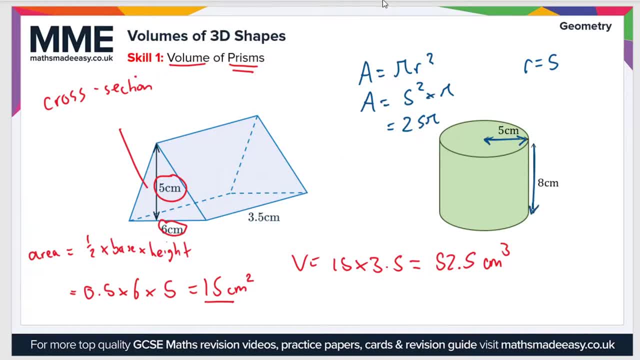 And then all we do to find the volume is we multiply that by the length or the height, which is 8cm. so the volume then is 8 times 25pi, which equals 200pi. Now, sometimes that would be ok if the question said: leave your answer in terms of pi, otherwise, 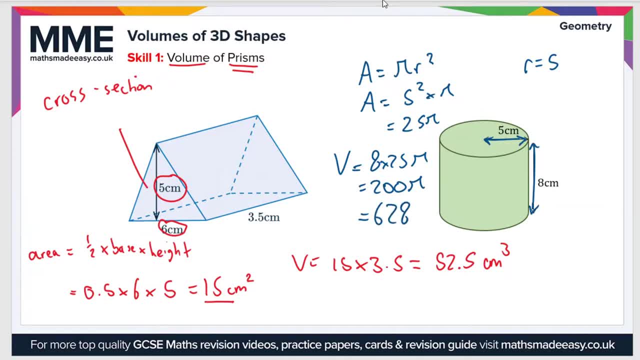 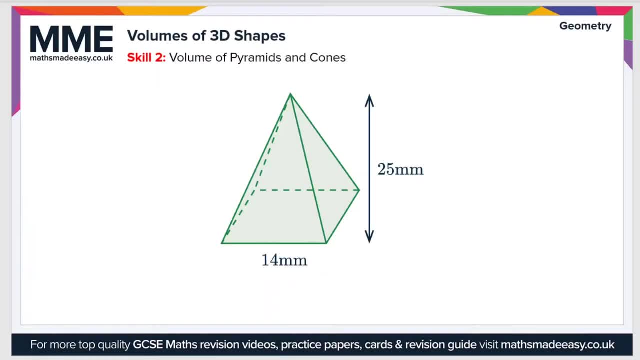 you could give it as a decimal, which is 628.3.. And the units would be centimetres, cubed again. So the second scale that we'll look at is calculating the volume of pyramids and cones. Now, the reason that these are grouped together is because a cone is essentially just a circle. 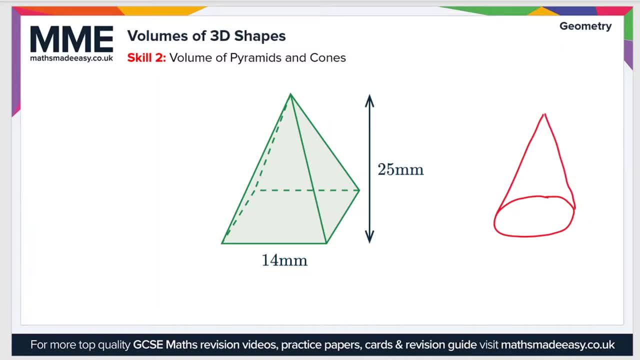 based pyramid, So the formula that you'll use is the same for both. So the formula that we need is volume equals 1 third times a. a is the area of the circle, a is the area of the base of the pyramid or cone. 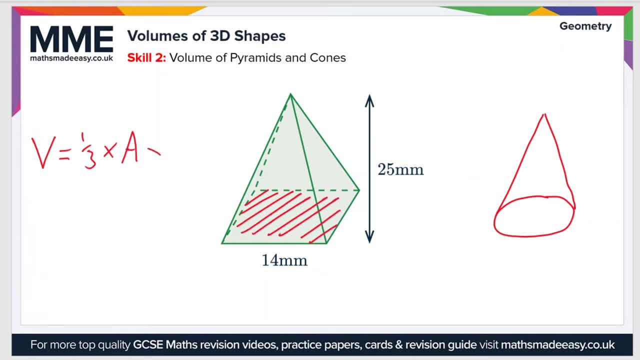 So in this pyramid here that would be the square base, And then we times that by the vertical height, So that would be that for the cone here it's given us 25 for the pyramid. So let's calculate the volume of the pyramid that's been given. 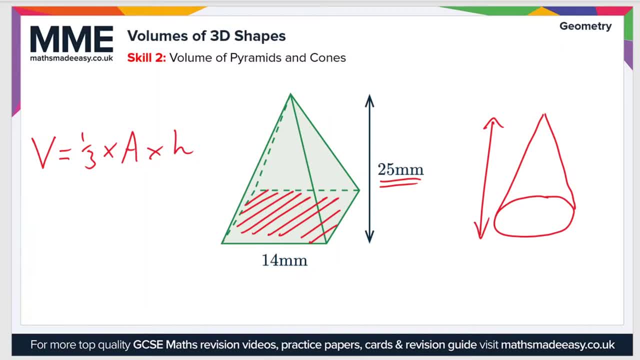 First of all, let's calculate the area of the base, So it's a square base pyramid. so that means that the other dimension is also 14mm. So a equals 14 times 14, or 14 squared, And that gives us a value of 196.. 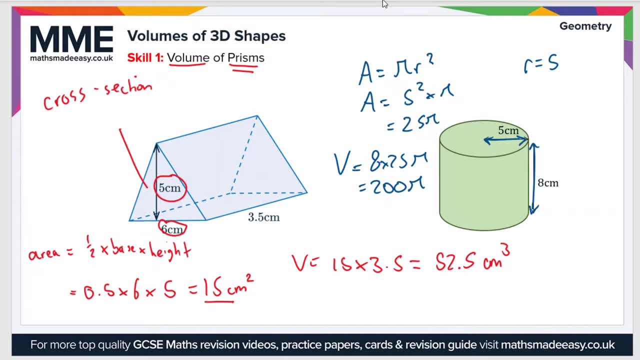 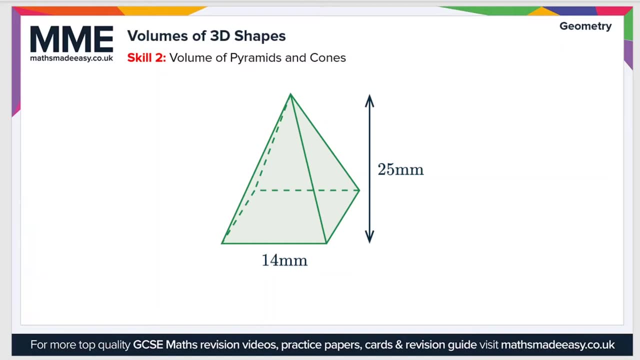 would be ok if the question said: leave your answer in terms of pi, otherwise you could give it as a decimal, which is 628.3, and the units would be centimetres cubed again. So the second scale that we'll look at is calculating the volume of pyramids and cones. Now the 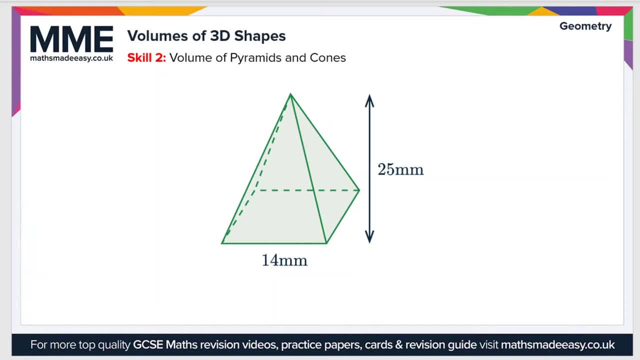 reason that these are grouped together is because a cone is essentially just a circle based pyramid, So the formula that you'll use is the same for both. So the formula that we need is: volume equals 1 third times a. Now a is the area of the base of the pyramid. 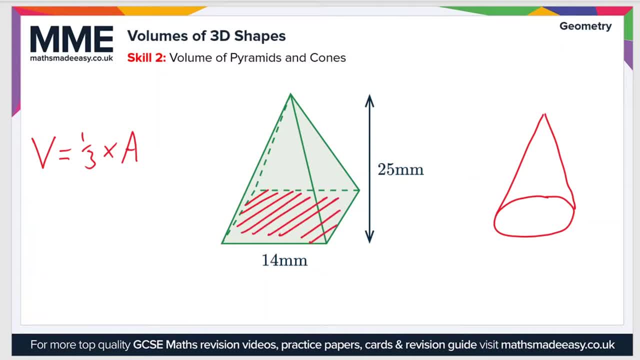 or cone. So in this pyramid here that would be the square base and then we times that by the vertical height. So that would be that for the cone Here it's given us 25 for the pyramid. So let's calculate the volume of the pyramid that's being given. First of all, let's calculate. 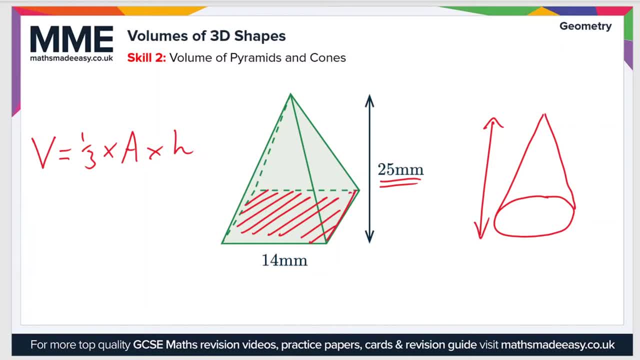 the area of the base. So it's a square based pyramid. so that means that the other dimension is also 14 millimetres. So a equals 14 times pi. So that's the volume of the pyramid that's being given. So that's 14 or 14 squared, and that gives us a value of 196.. Now the units would be: 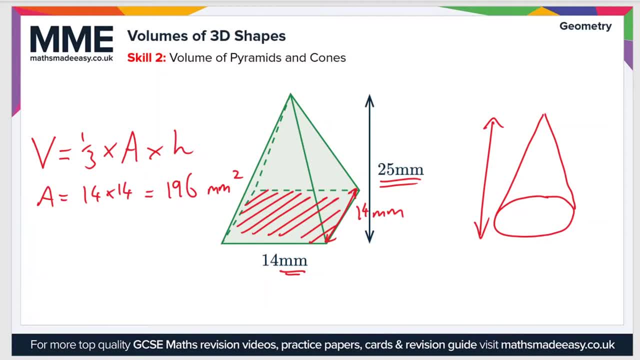 millimetres squared, because the units- sorry, the lengths- are given in millimetres. Okay, and then all we do to find the volume is we times our value of 196 by 1 third and by the vertical height, And if we do all that, it gives us a value of 1633.. 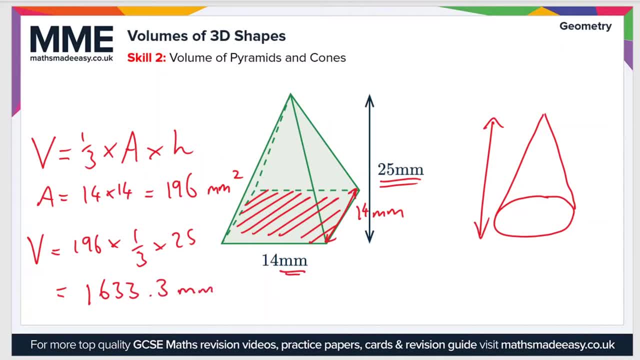 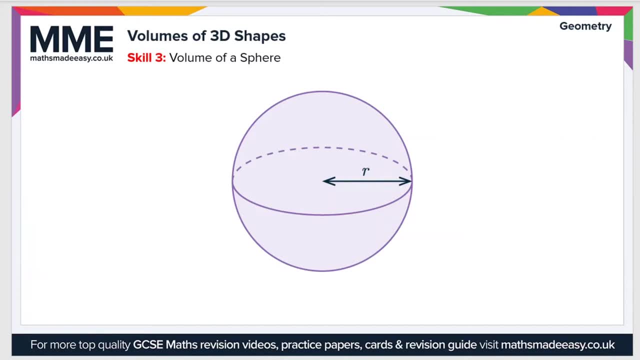 Okay, 0.3 millimetres cubed in this case. So the final skill that we'll look at in this video is calculating the volume of a sphere. Once again, it's a specific formula that we need, and the formula is: volume equals 4 divided. 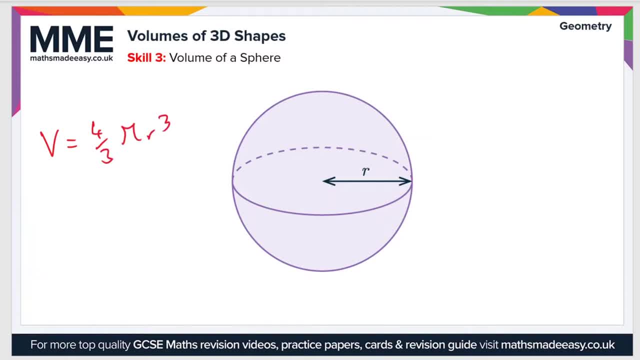 by 3 pi r cubed. So let's say that the value of r was 3.. If we plug these in to the formula, that would give us 4 over 3 pi times 3 cubed. So volume equals 4 divided by 3 pi times 27. and if you cancel that down you should get. 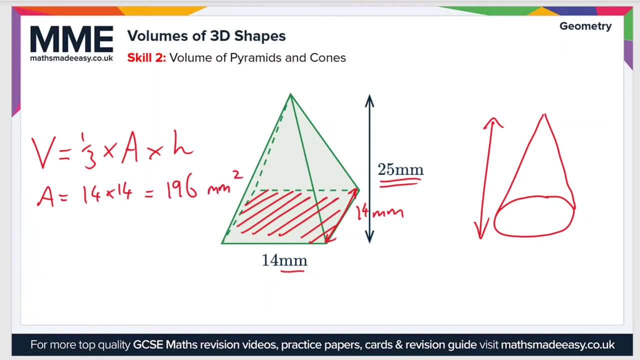 Now the units would be millimetres squared, because the lengths are given in millimetres. Ok, and then all we do to find the volume is we times our value of 196 by 1 third and by the vertical height, And if we do all that, it gives us a value. 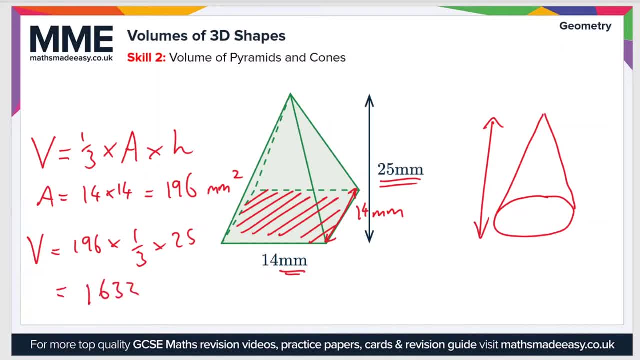 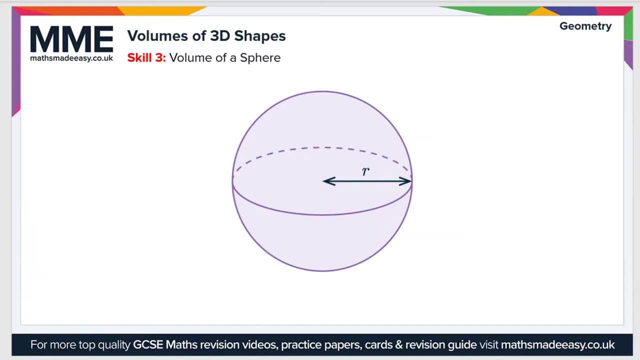 So that's the value of 196.5.. So that's the value of 1633.3 millimetres cubed in this case. So the final skill that we'll look at in this video is calculating the volume of a sphere. 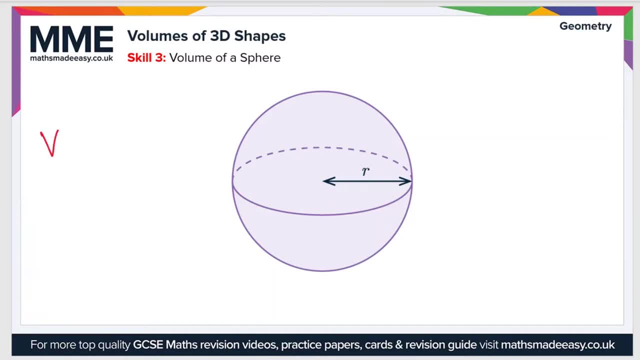 And once again it's a specific formula that we need, And the formula is: volume equals 4 divided by 3 pi r cubed. So let's say that the value of r was 3, if we plug these into the formula, that would: 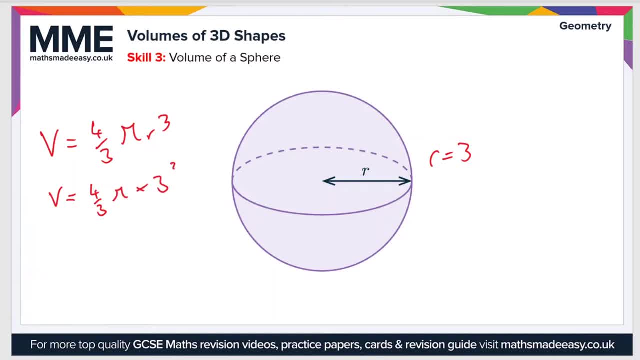 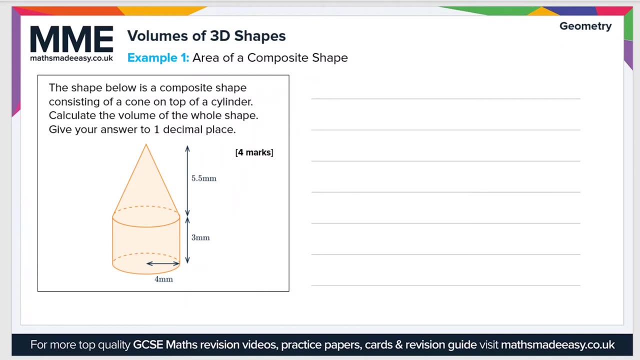 give us 4 over 3 pi r cubed, So volume equals 3 pi times 3 cubed. So volume equals 4 divided by 3 pi times 27.. And if you cancel that down you should get a value of 36 pi. 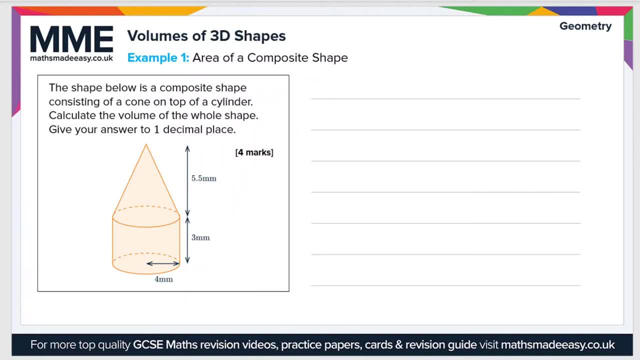 So let's have a look at an example question now. So the shape below is a composite shape consisting of a cone on top of a cylinder. Calculate the volume of the whole shape. Give your answer to one decimal place. So let's break this up and work out the volume of the cone. 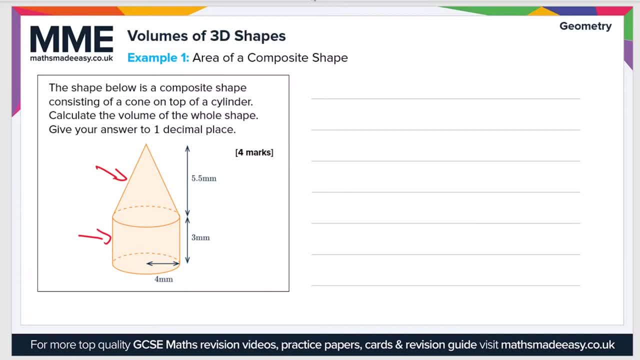 And then we'll work out the volume of the cone cylinder separately. So to work out the area of the cylinder, we first of all need the area of the circular base. So the area of the circle is pi? r squared and there r, in this case is four millimeters. 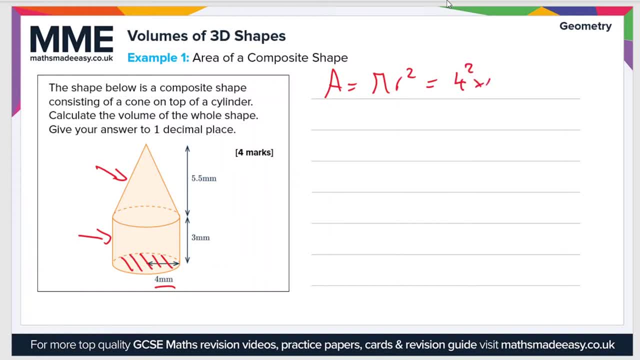 so the expression becomes four squared times pi, which is 16 pi, and the units will be millimeters squared. and then to work out the volume, let's say volume of the cylinder, all we have to do is multiply this 16 pi millimeter squared by the height, which is three millimeters. 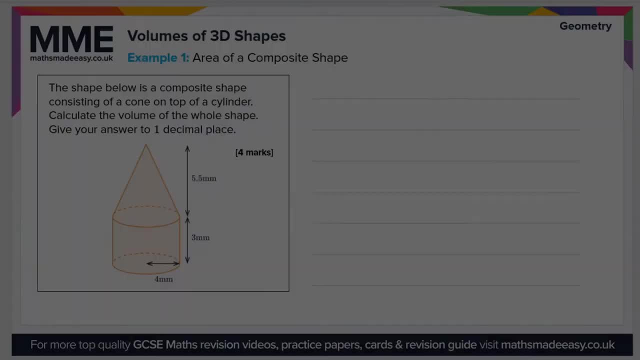 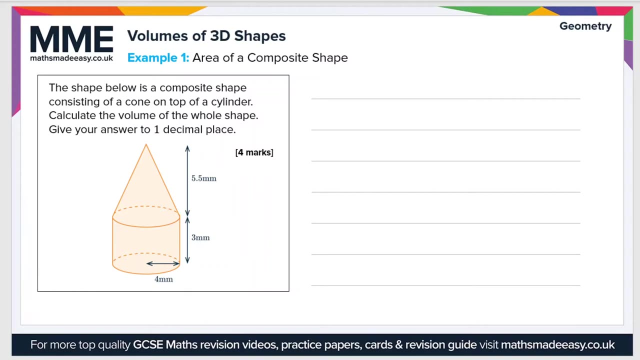 a value of 36 pi. So let's have a look at an example question now. So the shape below is a composite shape consisting of a cone on top of a cylinder. Calculate the volume of the whole shape. Give your answer to one decimal place. 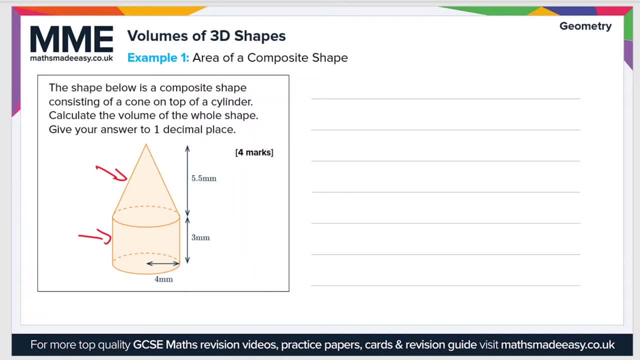 So let's break this up and work out the volume of the cone and the cylinder separately. So So, to work out the area of the cylinder, we first of all need the area of the circular base. So the area of the circle is pi? r squared and there r, in this case is 4mm. 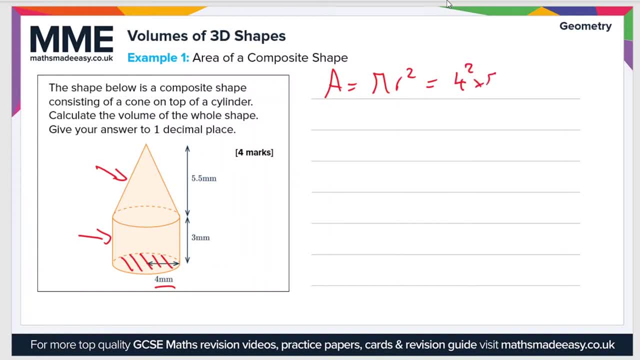 So the expression becomes 4 squared times pi, which is 16pi, and the units will be mm2.. And then to work out the volume, let's say volume of the cylinder, all we have to do is multiply this 16pi mm2 by the height, which is 3mm. 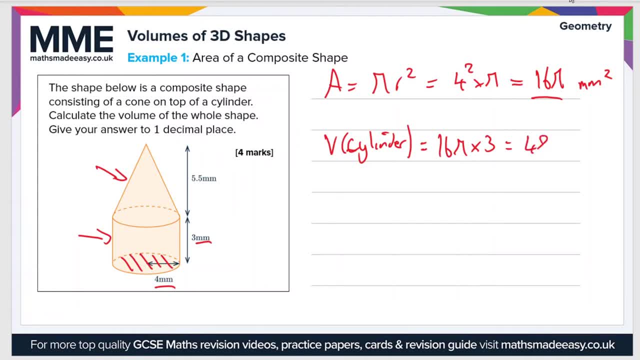 So 16pi times 3 and that gives us 48pi mm3 for the volume of the cylinder, Now the volume of a cone, we use the formula which is third times the area of the base, which in this case we've already worked out as 16pi, and then we times that by the height. 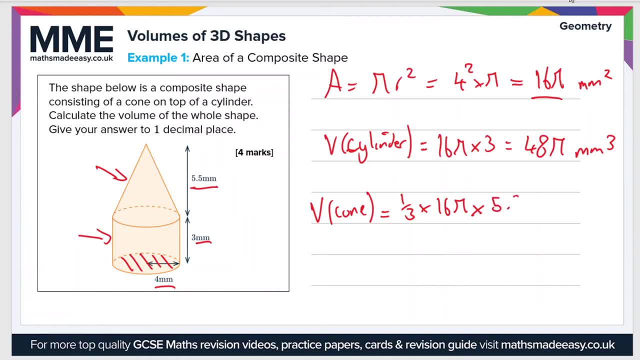 of the cone, which is 5.5mm. And if we plug all that into the calculator it gives us a value of 88 over 3pi mm3.. So that's the volume of the cone and the total volume. call it: vtotal is just 48pi. so the 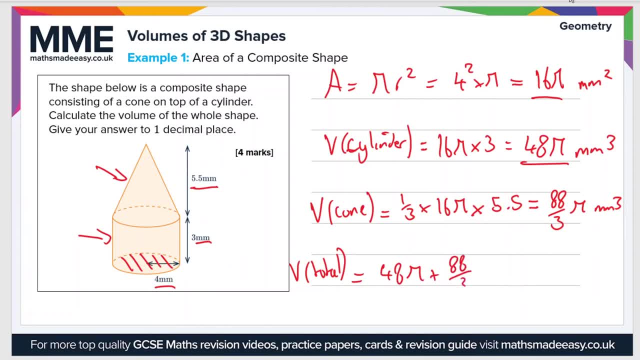 volume of the cylinder plus 88 over 3pi, which is the volume of the cone. Now if we plug all that into the calculator, it gives us a value of 242.945.. So that's the volume of the cone. Or to one decimal place, that's what your question asks for, that's 242.9, and then the 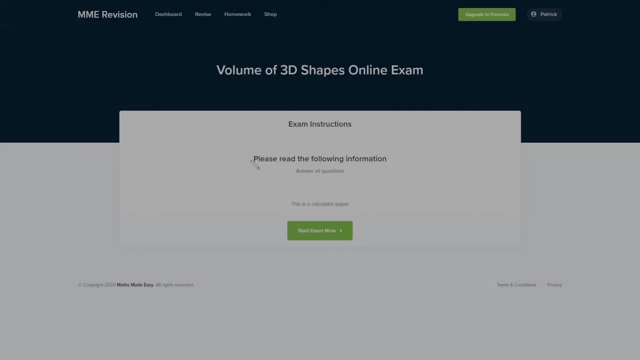 units will be mm3.. So if you'd like to improve at this topic or just practice some exam style questions, then we do have an online exam available on the volumes of 3D shapes. You can find it through our revision platform. so if you click the link it will take you.